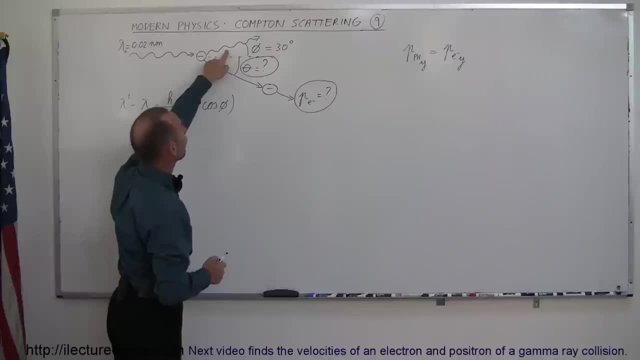 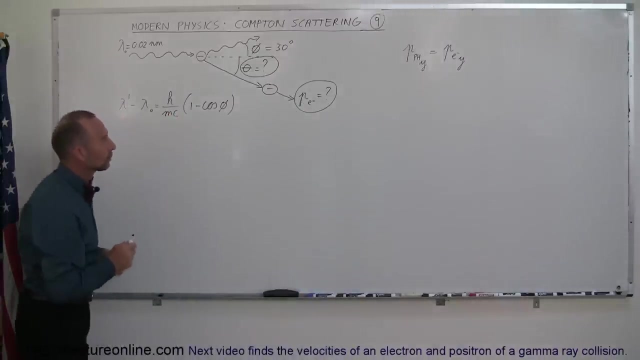 means the component of the momentum of the photon after the collision in the y direction should be equal in magnitude to the component of the momentum of the electron in the y direction, of course, after the collision. And that's what we have up here on this equation that the momentum in the y direction should cancel out. All right, so strategy First, we're going to find the scattered angle of the photon. From that we'll calculate the change in the energy which is then imparted on the electron. 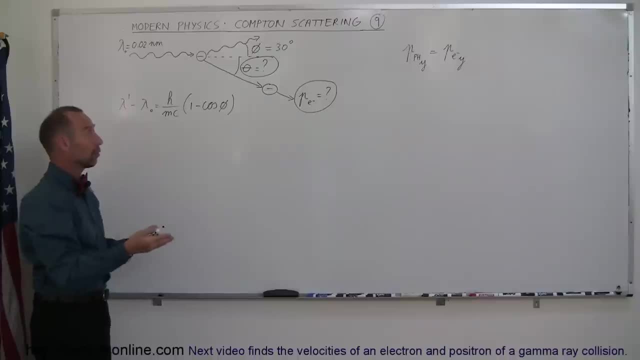 That means we'll be able to find the kinetic energy of the electron, and henceforth we'll be able to find the velocity of the electron. and if we know the velocity of the electron, we'll be able to find the momentum of the electron. and then, finally, we should be able to figure out the angle by using conservation of momentum. Seems like a lot of things to do here, but let's just take it one step at a time. So the first step should be straightforward: Let's find the new wavelength of the scattered photon, and so it would be equal to the original wavelength. we move it across the equal sign plus h over mc times. 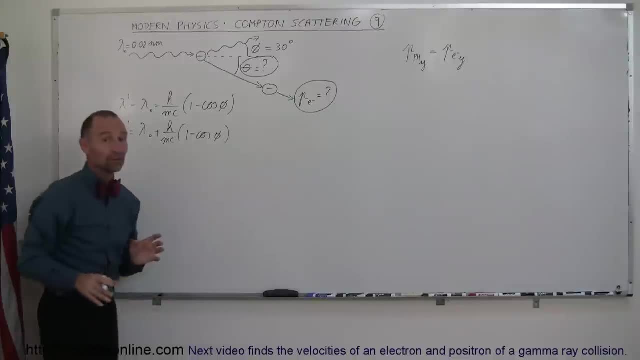 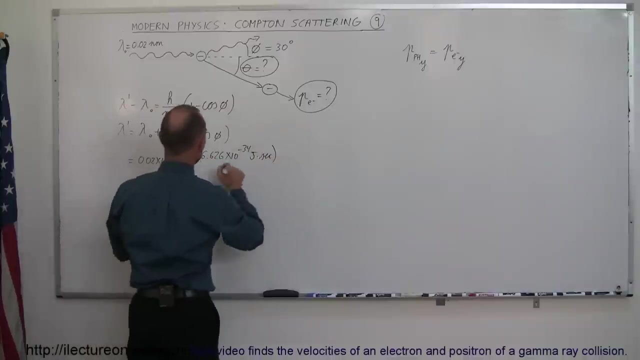 1 minus the cosine of phi. So this by now, if you've watched the video, should become familiar to you. Let's plug in the numbers. assuming that the original wavelength was 0.02 times 10 to the minus 9 meters plus h, which is 6.626 times 10 to the minus 34 joules times seconds multiplied by times no divided by the mass: 9.11 times 10 to the minus 31. 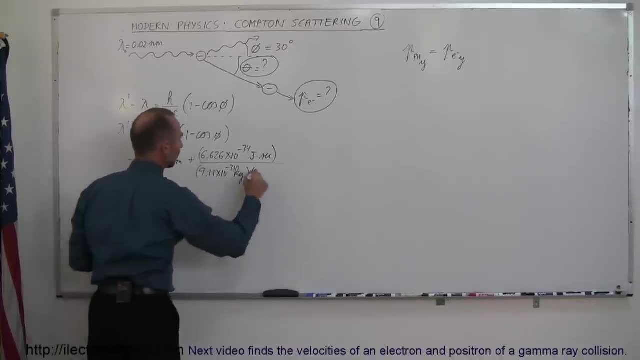 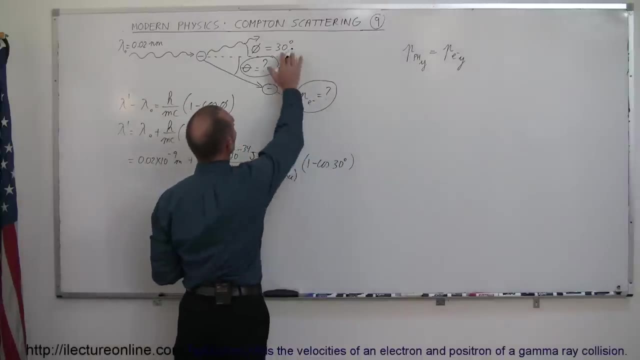 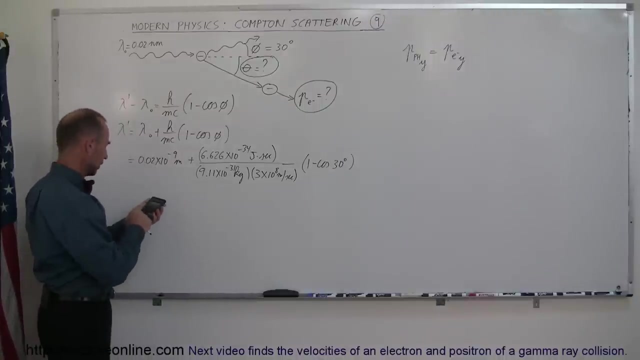 kilograms, that's the mass of an electron multiplied by times the speed of light and finally, multiplied by times 1 minus the cosine of the scattered angle, which we assume to be 30 degrees in this case. So we're talking about the scattered angle of the photon, Alright, so what is that? equal to? So 6.626 e to the 34 minus divided by 9.11 e to the 31 minus divided by 3 e to the 8.. 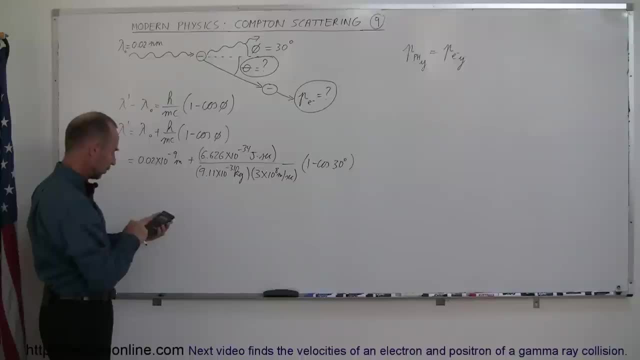 Multiply that times 1 minus the cosine of 30, equals, and then add that to 0.02 e to the 9 minus equals, and so this now becomes 2.0325 times 10 to the minus 11 meters. So that's the new wavelength. Notice that this would be 2 times 10 to the minus 11, so it's a little bit bigger than it was before the effect was made. 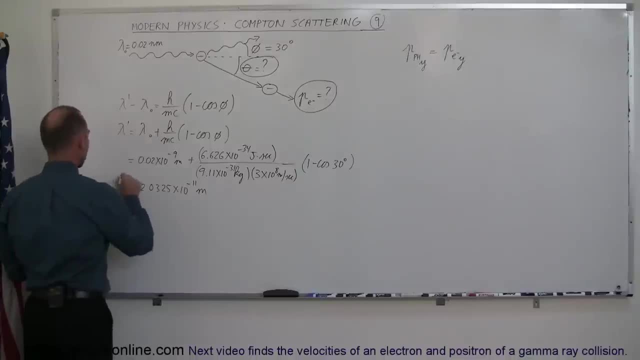 The photon got scattered off. So if that's now the final wavelength after the collision, now we're going to find the change in the energy. So the change in the energy is equal to the energy initial minus energy final. The initial energy would be h times the frequency initial minus h times the frequency final, And of course the frequency can be written as c over lambda, so this would be: 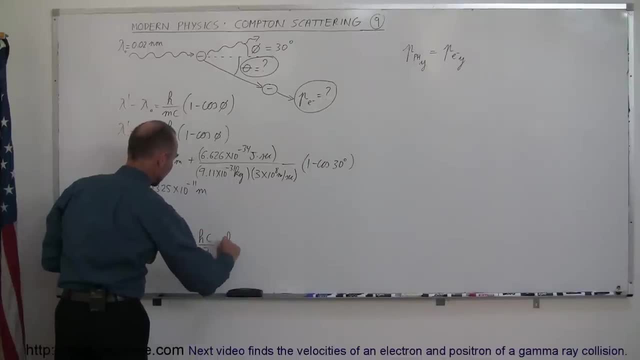 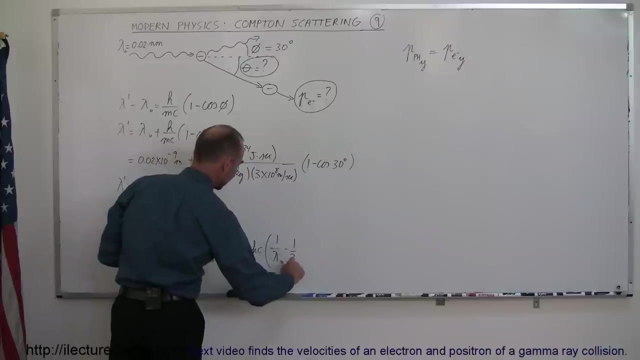 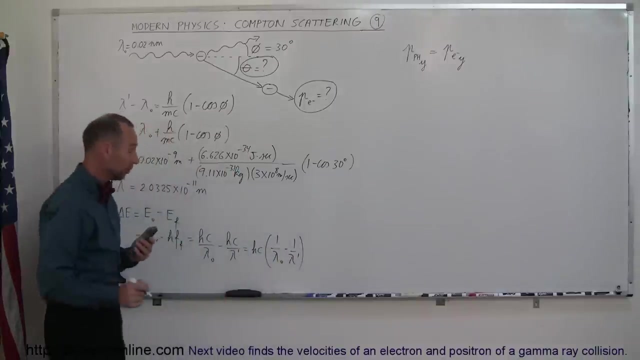 equal to hc over lambda initial minus hc over lambda final, And so final lambda was lambda prime And so, factoring out an hc, this can be written as h times c times 1 over lambda initial minus 1 over lambda final, And that's a lousy-looking lambda. so let me write that again. There we go. Now plug in the numbers. 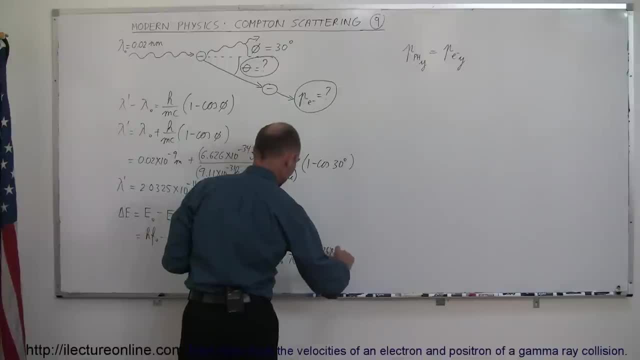 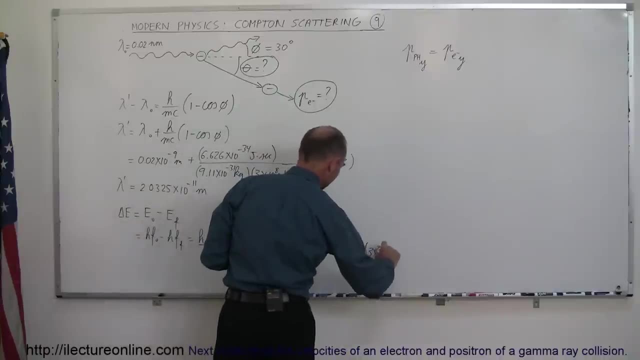 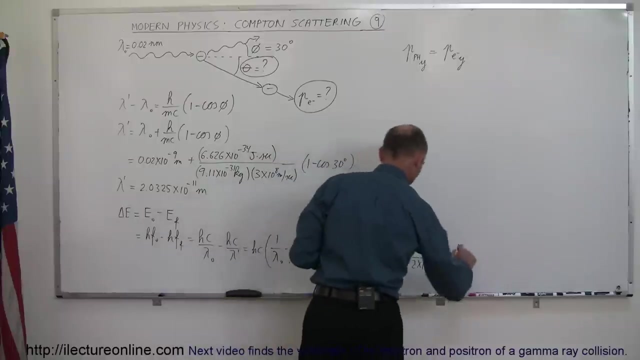 This is equal to 6.626 times 10 to the minus 11 meters, Minus 34 Joules times seconds. Speed of light: 3 times 10 to the 8 meters per second. Forgot the 8 there. All right, Now we multiply it times 1 over lambda initial, so 1 over 2 times 10 to the minus 11.. That would be meters minus 1 over 2.0325.. 0325 times 10 to the minus 11 meters. 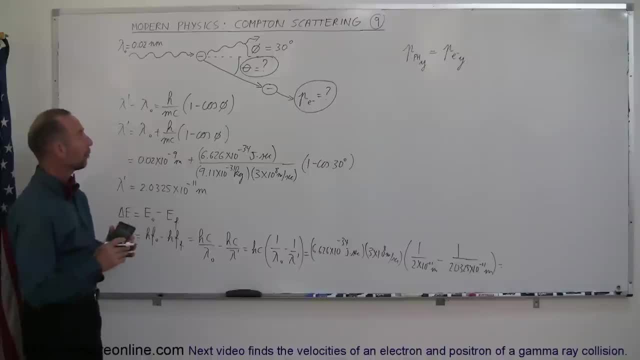 And that will give us the change in the energy of the photon before the collision and after the collision. All right, So 1 divided by 2 e to the 11 minus minus 1 divided by 2.0325 e to the 11 minus equals. All right, So now we multiply it times the speed of light, times 3 e to the 8.. 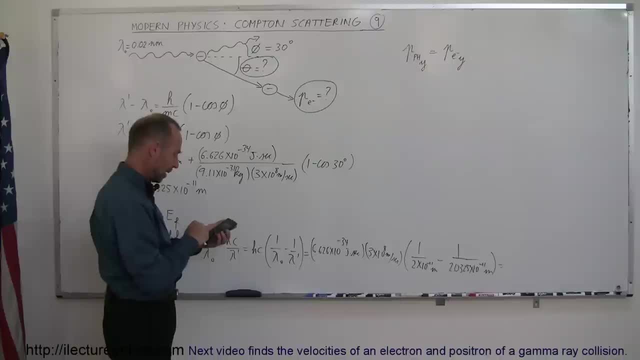 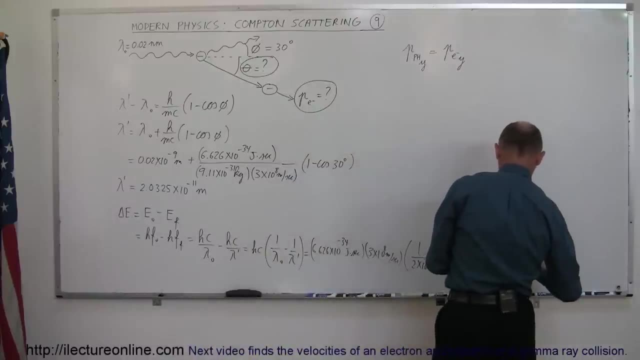 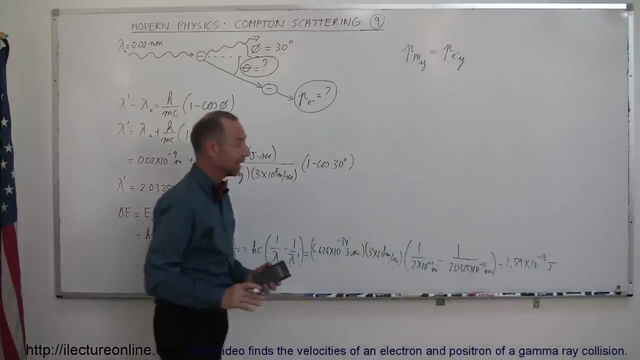 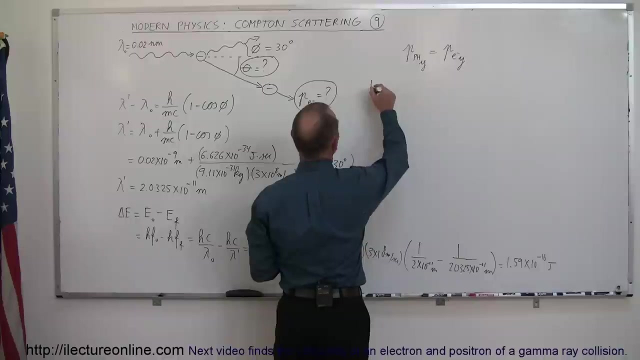 And times 6.626 e to the 34 minus, And I get 1.59 times 10 to the minus 16 Joules. So that's the change in the energy of the photon. Of course that energy is imparted onto the electron, So let's do that. We then say that the kinetic energy is equal to one half mv squared. which means that the kinetic energy is equal to one half mv squared. 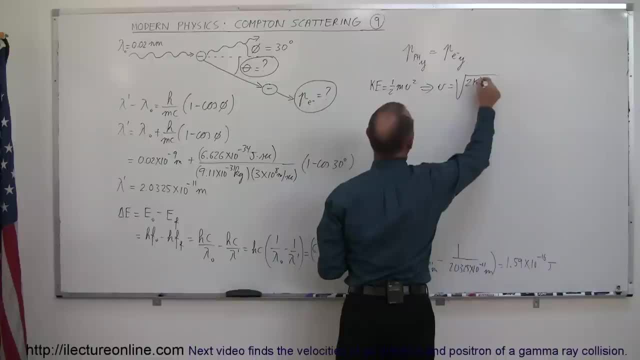 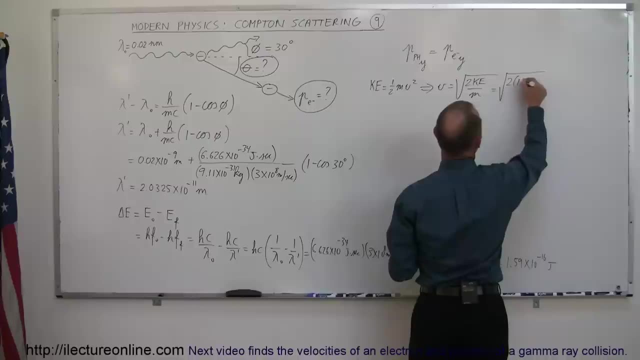 So that means that v is equal to the square root of 2 times the kinetic energy divided by the mass, which is equal to the square root of 2 times the kinetic energy. we have here 1.59 times 10 to the minus 16 Joules, all divided by the mass, 9.11 times 10 to the minus 31 kilograms. 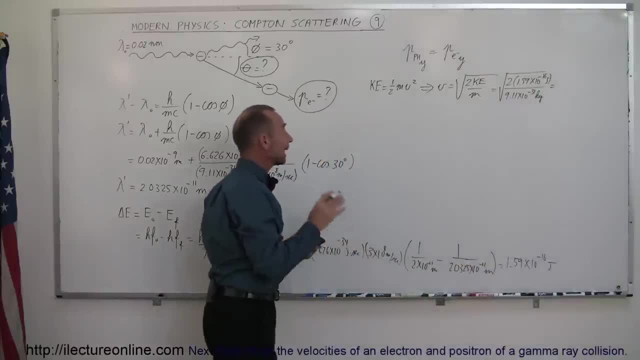 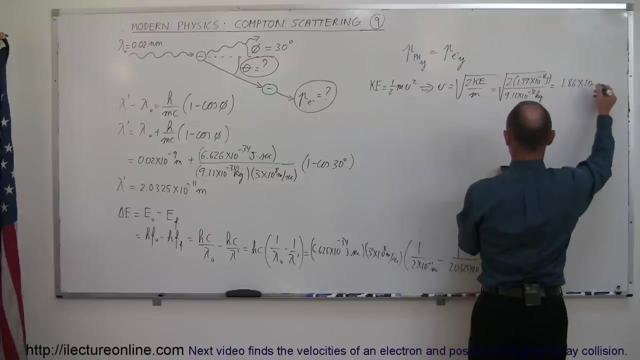 So that will give us the velocity of the electron after the collision, because remember that all of the energy that the photon lost was given to the electron. So we multiply that times 2 and divide it by 9.11- e to the 31 minus equals, and take the square root And this is 1.86 times 10 to the 7th, I believe. Let me check. 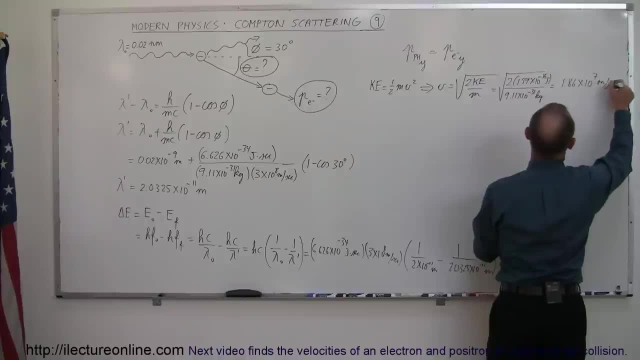 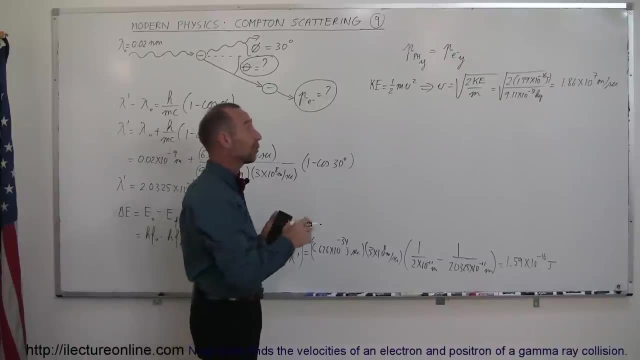 Sure thing, Yeah, 1.8 times 10 to the 7 meters per second, which is about 6% of the speed of light, which makes it still non-relativistic. You always want to check for that. If it's relativistic, you want to check for that. 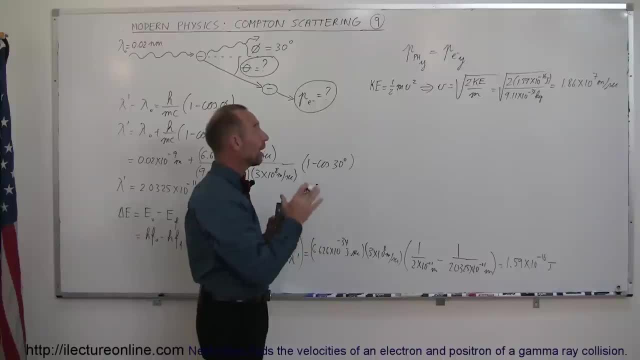 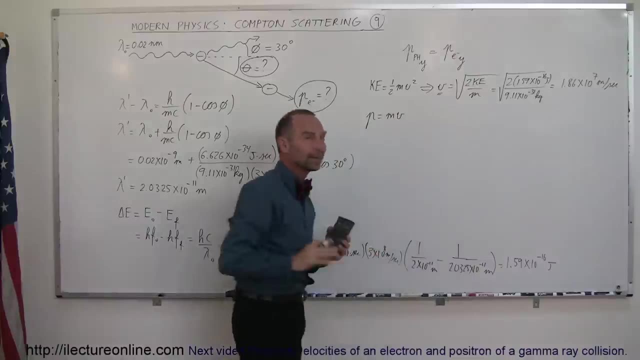 You want to do things a little bit differently? All right. now that we know the velocity of the electron, now we can say that the momentum p is equal to mv. We don't have to worry about the gamma, the relativistic effect. 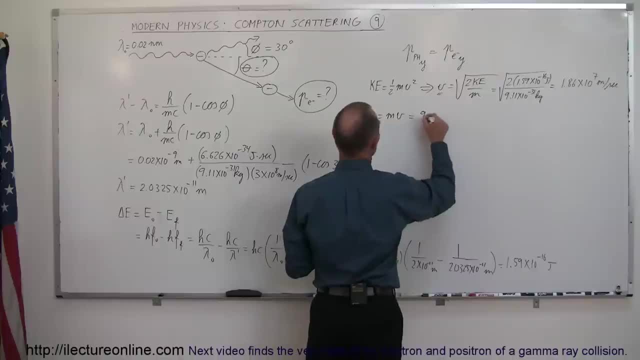 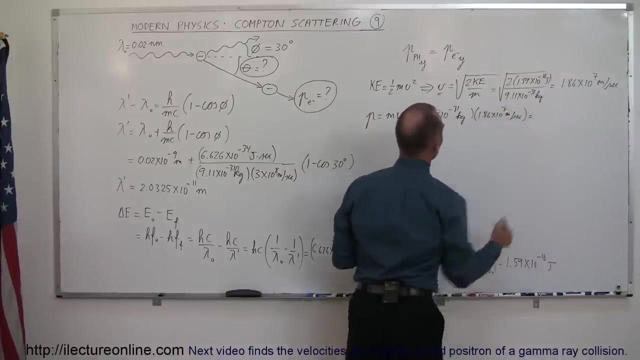 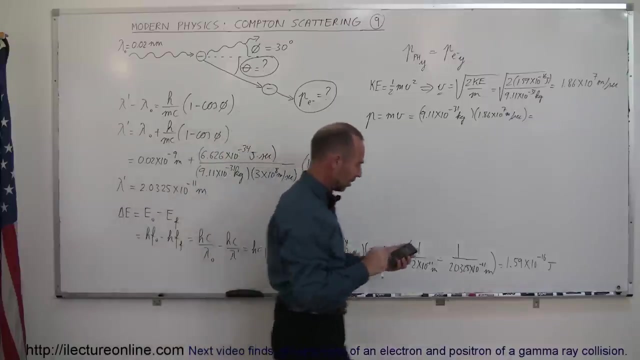 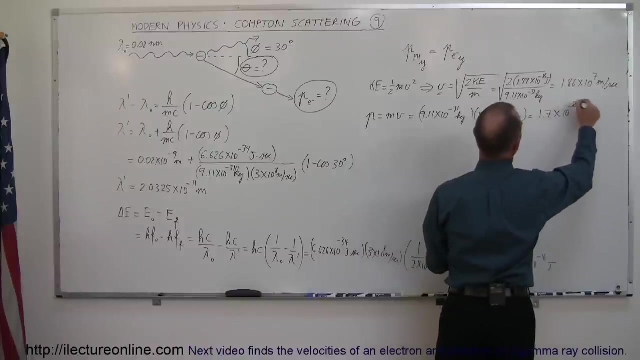 So this is equal to the mass, which is 9.11 times 10 to the minus 11, minus 31 kilograms times velocity, which is 1.86 times 10 to the 7th meters per second. So times 9.11 e to the 31 minus equals, and that gives us 1.7 times 10 to the minus 23 kilograms meters per second. 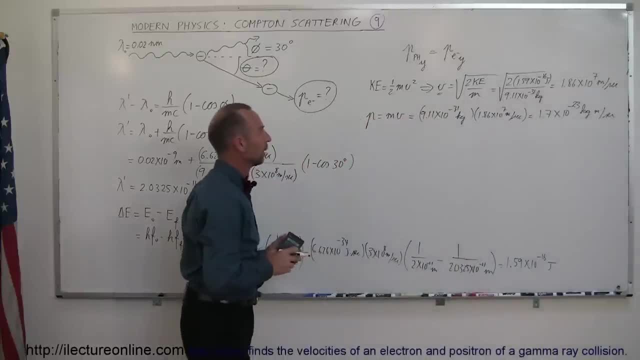 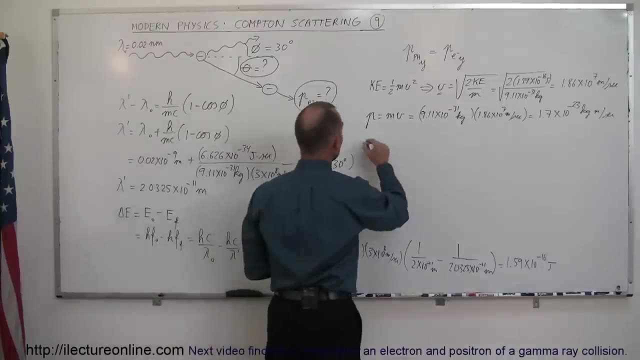 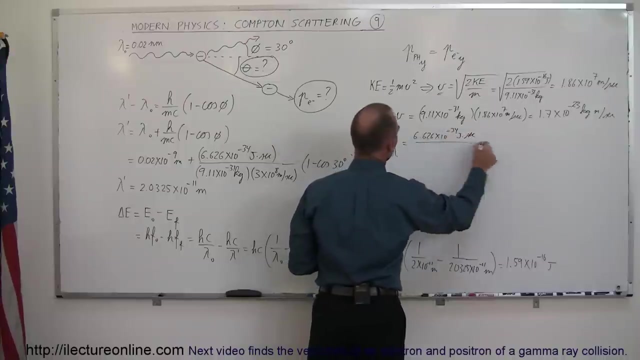 All right, now we have the momentum of the electron, Now we want to get the momentum of the photon. Remember the momentum of the photon, p of a photon. It's simply equal to h over lambda. So that would be equal to 6.626 times 10, to the minus 34 joules times seconds divided by lambda. 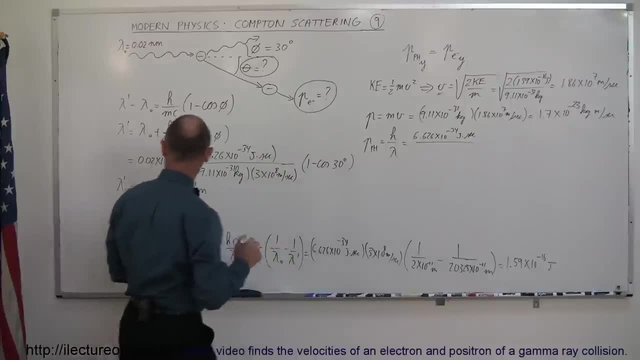 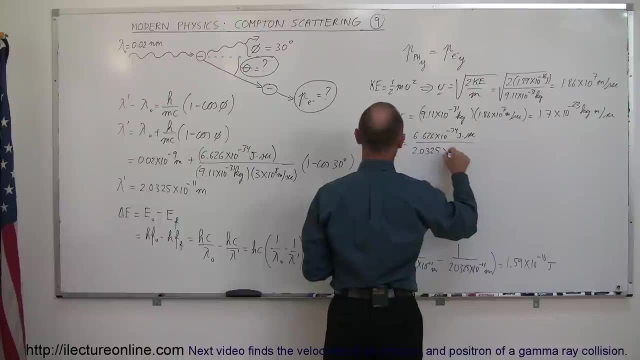 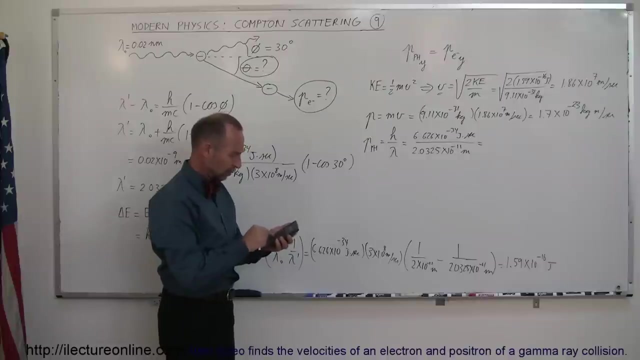 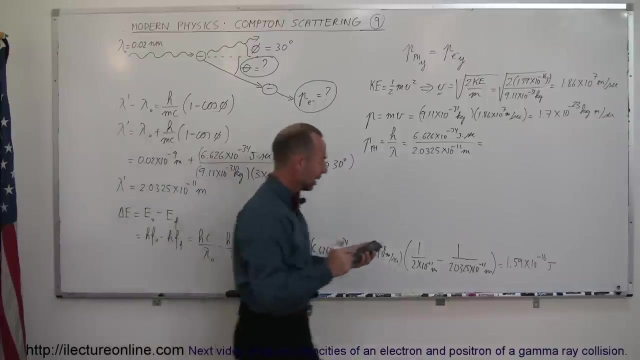 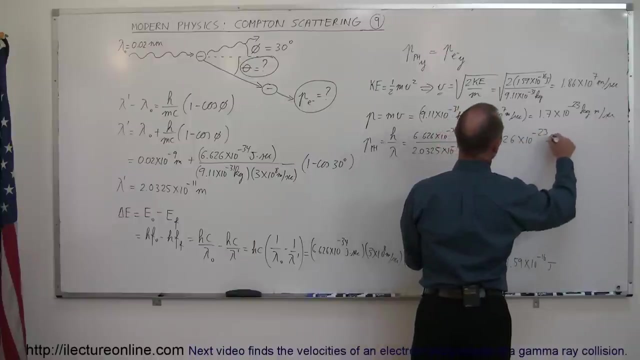 And lambda of the eventual photon. that's right here. that would be this one right here. So that would be 2.0325 times 10 to the minus 11 meters. And so let's do that: 6.626 e to the 34 minus divided by 2.0325 e to the 11 minus equals, and we get 3.26 times 10 to the minus 23 kilograms meters per second. 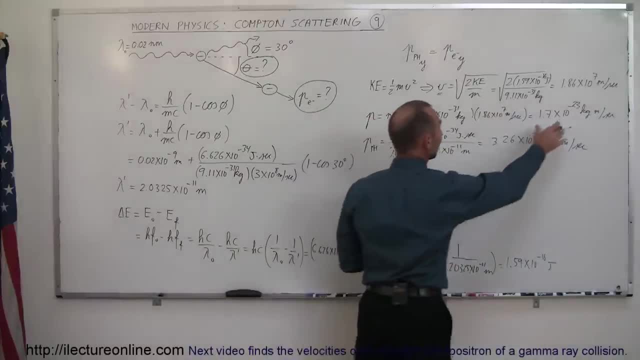 Now notice that the momentum of the electron and the momentum of the photon are kind of the same right. So you can see here the momentum of the photon is only about twice as much As the momentum of the electron. So that at least tells you we're in the ballpark here. 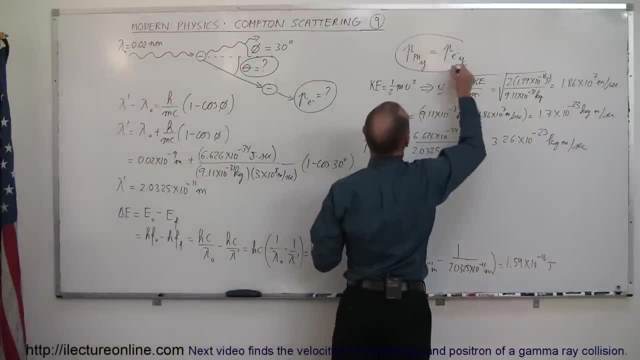 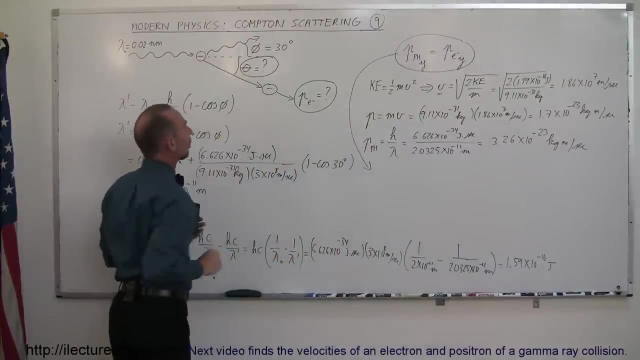 Now, the last thing we're going to do is we're going to set these two equal to each other, right? We're going to set the y components of each equal to each other, which allows us then to find the scatter angle of the electron. 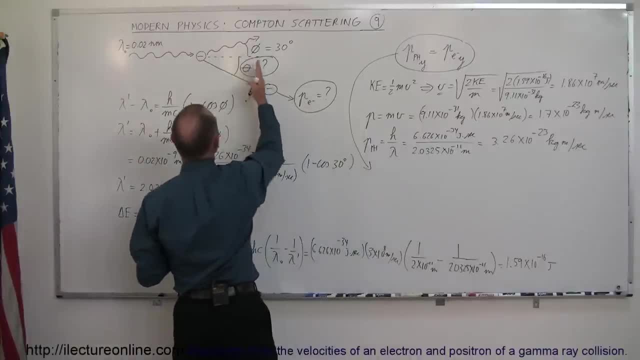 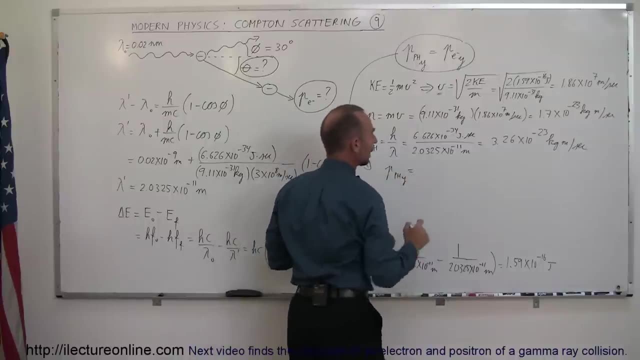 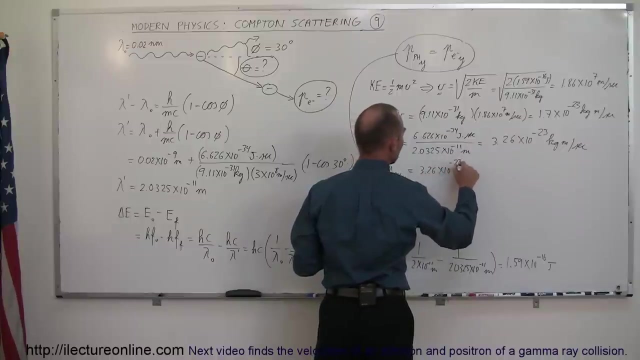 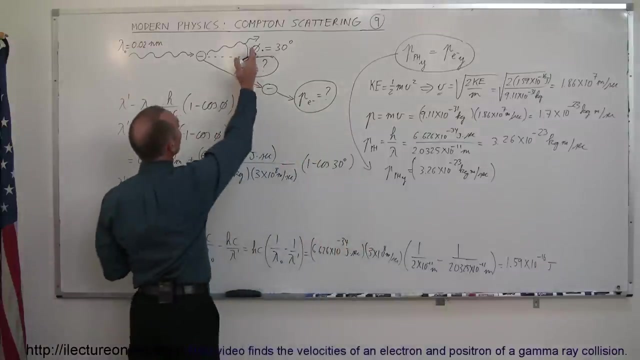 So, first of all, the momentum of the photon in the y direction. So p of the photon in the y direction is equal to that would be the momentum of the photon right here, That would be 3.2.. 6.626 times 10 to the minus 23 kilogram meters per second, and we multiply that times the y component of the momentum. 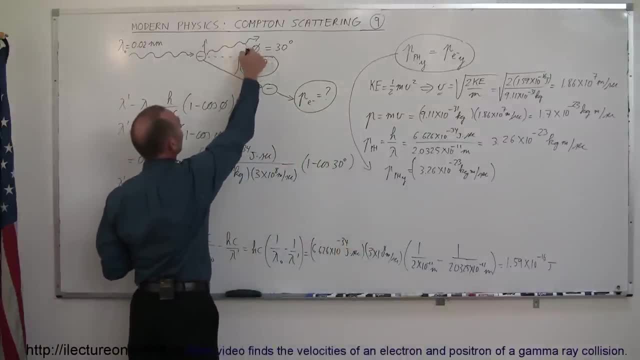 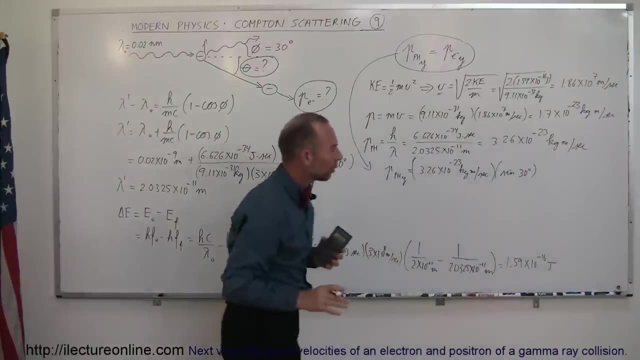 and the y component, of course, would be the opposite of the angle, which would be the sine of the angle of 30 degrees. So times the sine of 30 degrees, that gives us the y component of the electron momentum, or I should say the, not the electron but the photon momentum. 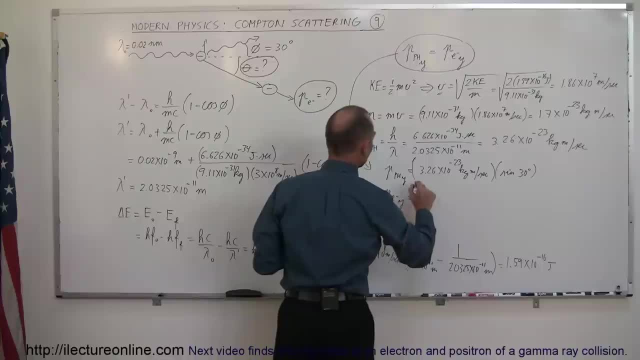 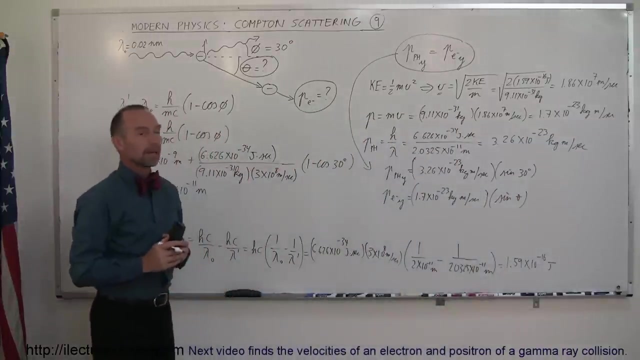 And so p of the electron in the y direction is equal to the momentum, 1.7 times 10, to the minus 23 kilogram meters per second. and then we have to multiply that times the sine of theta, And then we set those two equal to each other. When we do, 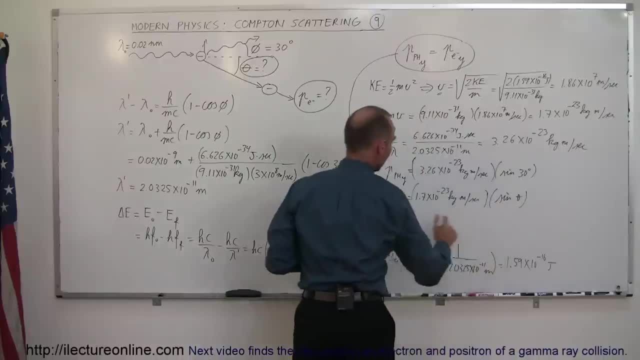 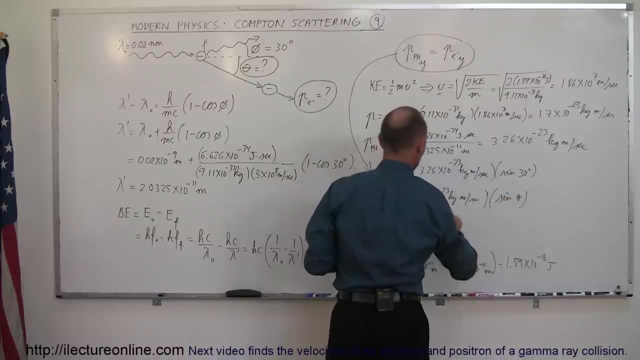 when this is equal to this. we're looking for the sine of theta. so we can say, then, that the sine of theta is equal to this divided by this. so that would be 1.26 times 10 to the minus 23,. divided by 1.7 times 10 to the minus 23, times the sine of 30 degrees. 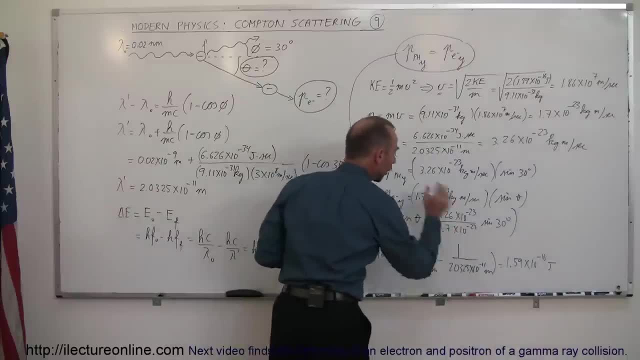 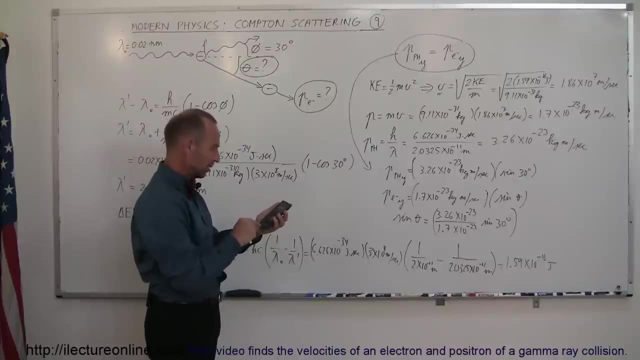 And then, of course, to find theta, we have to take the arcsine of that. Okay, so let's do that. So, divided by 1.7 e to the 23 minus, then times the sine of 30, and then we take the inverse of that. 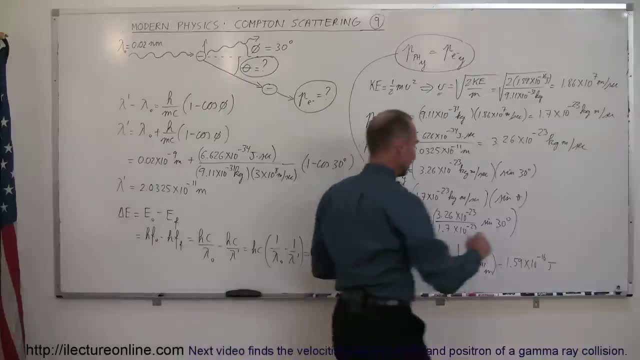 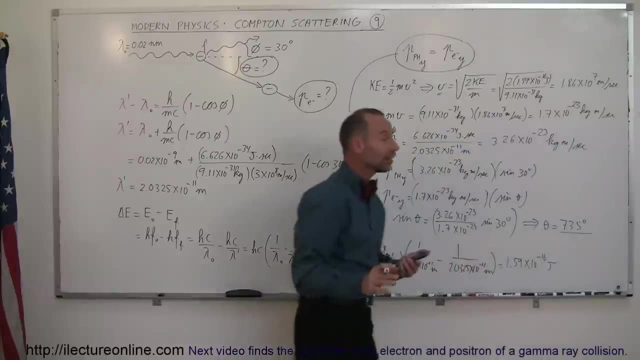 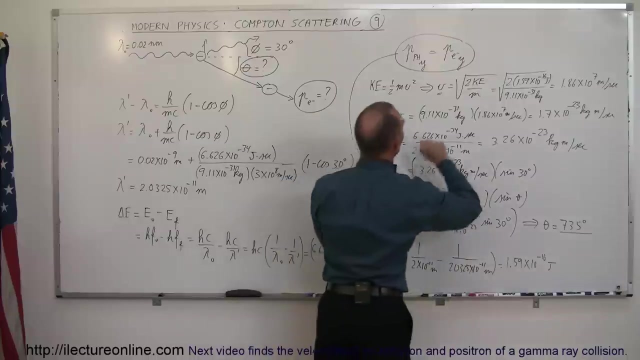 and that indicates, then, that theta is equal to 73.5 degrees, which is the scatter angle of the electron. So we were able to find the velocity of the electron right here. So the velocity of the electron is equal to this. That allows us to find the momentum of the electron, which is equal to mv. 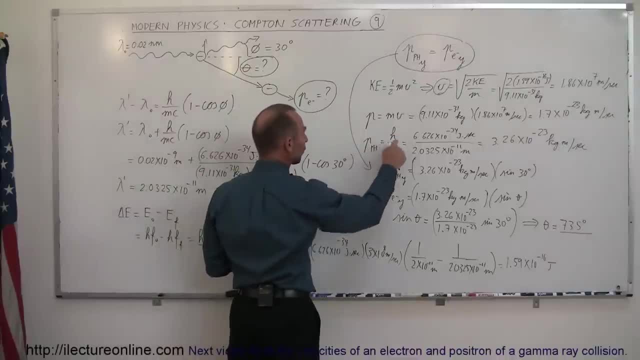 Then we notice that the momentum of the photon is h over lambda. Notice that the two are relatively similar, which is good. Now we can say that the y component of the momentum of the photon should equal the y component of the momentum of the electron. We set them equal to each other. 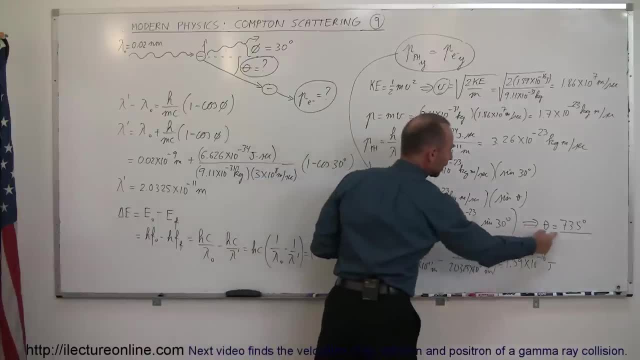 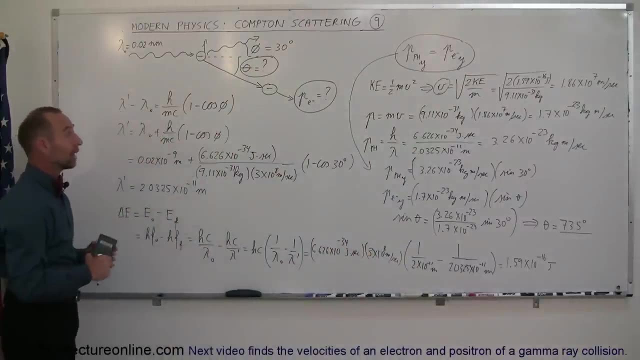 solve for sine of theta and then take the arcsine of theta, arcsine of this quantity to find theta. and theta happened to be 73.5 degrees. So that allows us to find the scatter angle of the electron. So you can see that using the Compton scattering you can find the changed wavelength. 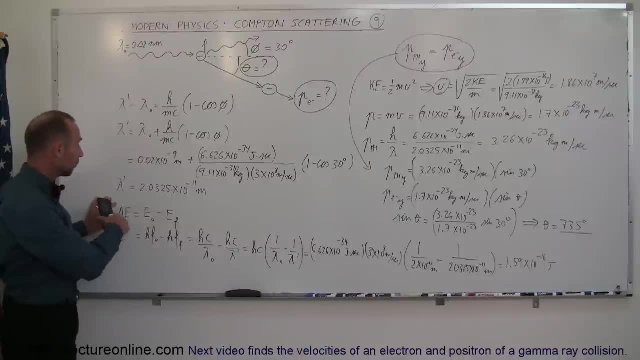 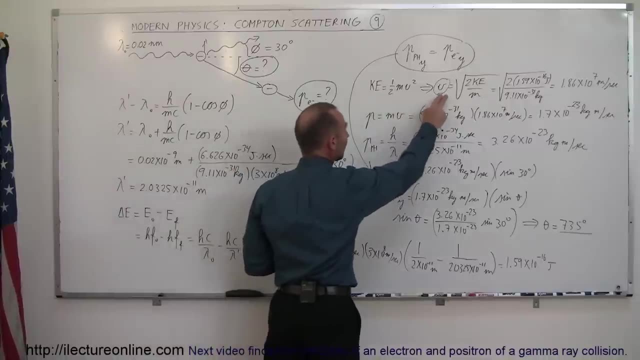 you can find the changed energy of the electron, of the photon, which means you can find the changed energy of the electron, which of course is kinetic energy. From that we can find the velocity, from that we can find the momentum, and from that we can find